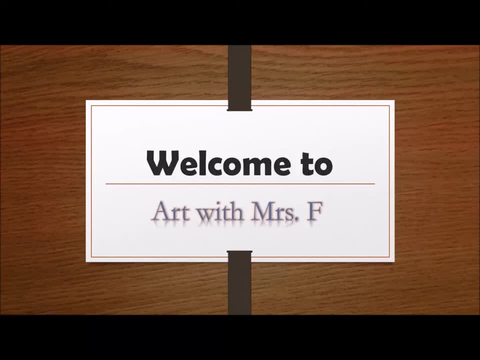 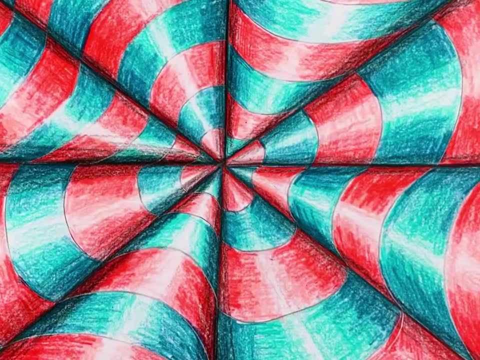 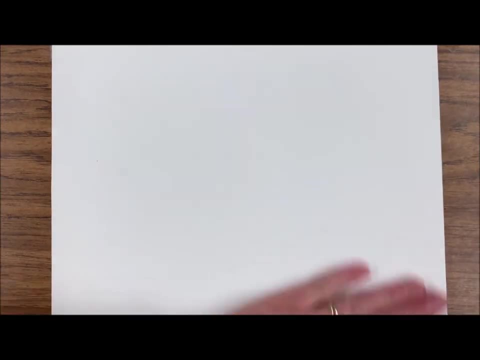 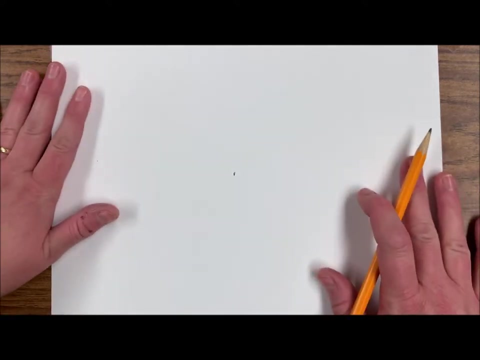 Hey guys, today we are going to be creating some op art using a few of these tools. So, starting with your blank piece of paper, we're going to make a dot in the center And then we are going to create about probably eight to ten sections using the ruler You want. 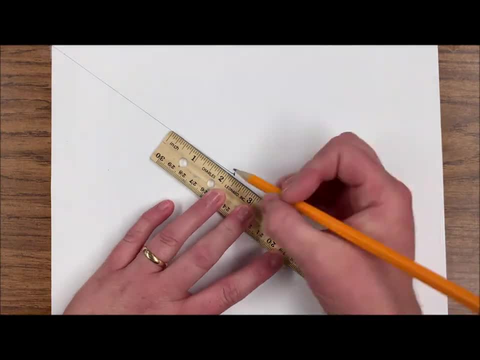 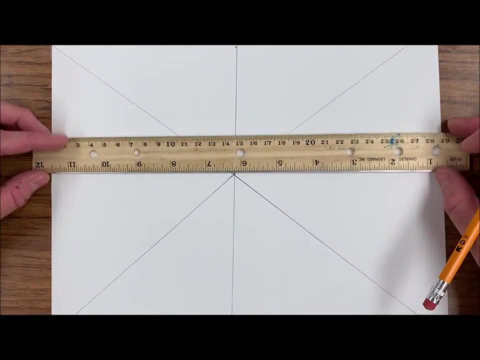 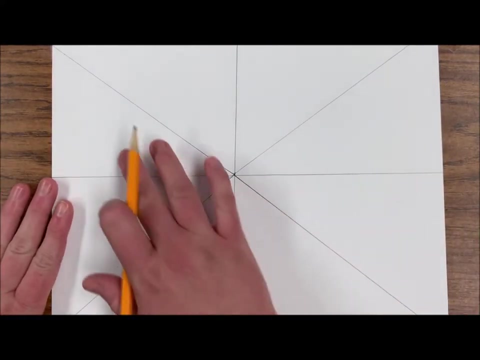 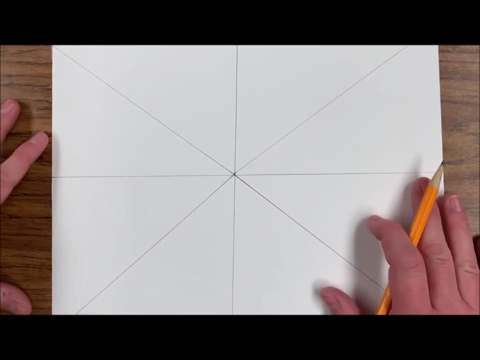 to go from the dot. Now that I've used my ruler to section off, I have one, two, three, four, five, six, seven, eight sections. You could do more or less. I feel like this is a good time to do it again, So in each of these I'm going to do circles. For the first, 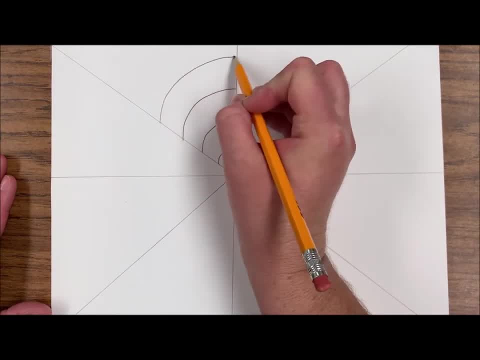 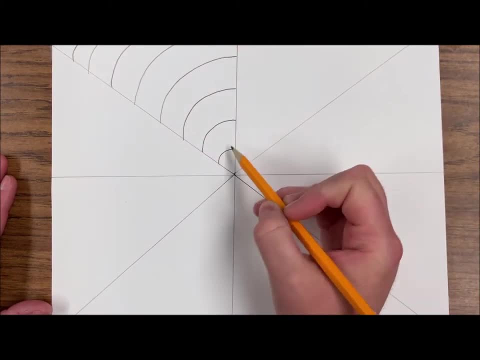 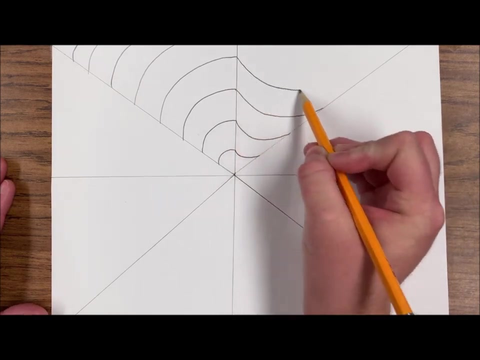 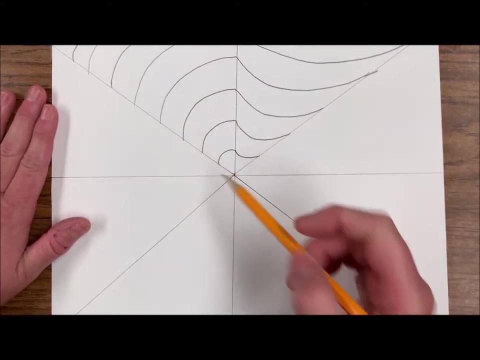 one I'm going to curve up, And for the ones next to it, I'm going to start from the same place, but for these ones I'm curving down. Continue this pattern: up, down, up down all the way around. 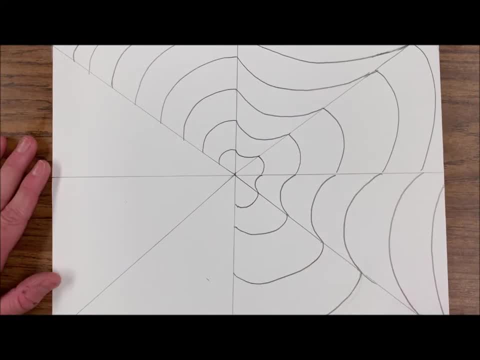 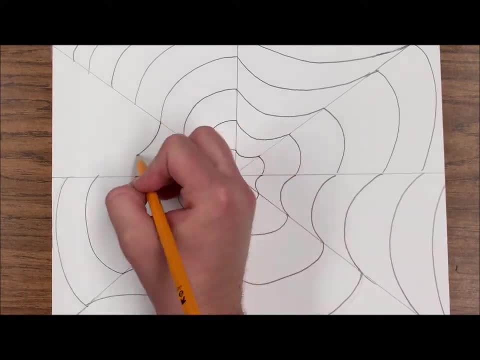 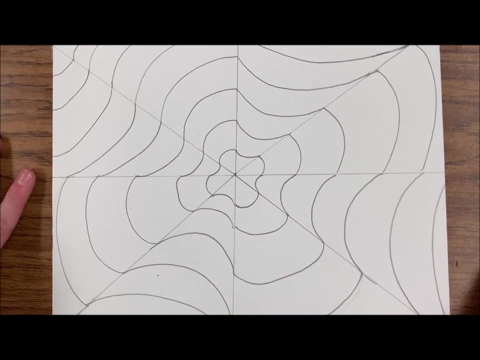 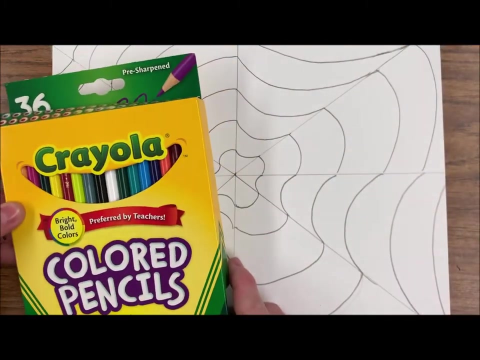 Once you've completed and connected them, they should have kind of a wavy pattern where they're all connected. Now the fun part is shading so that they look 3D. The key to shading is when you use your colored pencil. you want to shade harder along the edges and softer 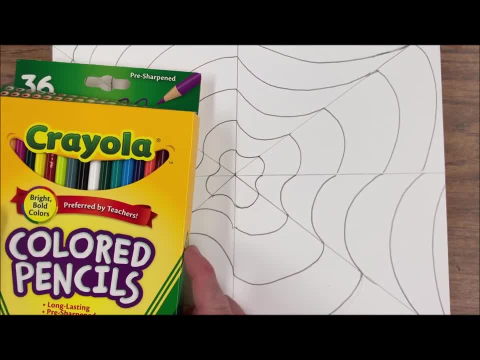 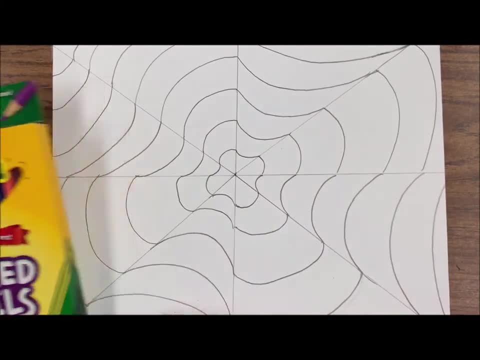 or lighter in the center. So you want to shade the edges of the pencil. So you want to shade the edges of the pencil and apply a little bit of shade on the edges of the pencil. You want to shade them where you don't want to shade them. You want to stay in the middle. 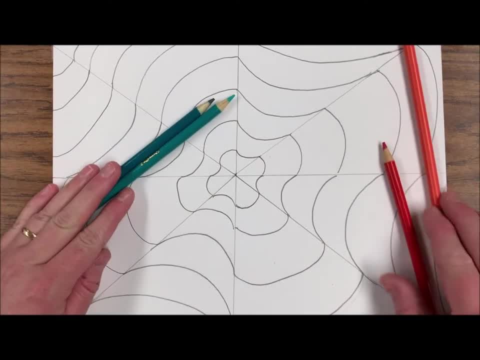 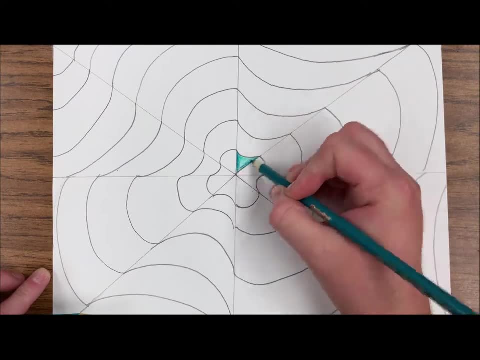 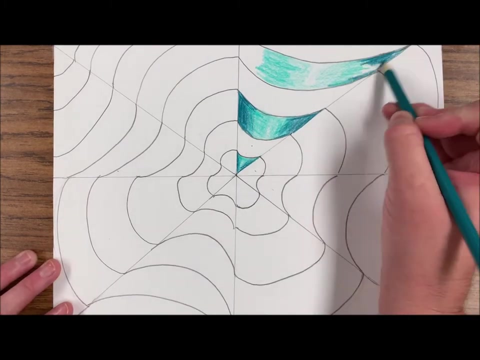 of the pencil, because the colored pencil is all about pressure. You want it to be harder on the edges and softer in the center, leaving a little bit of white in the very center For my colors. I'm going to be using colored pencils and I'm going to alternate warm and 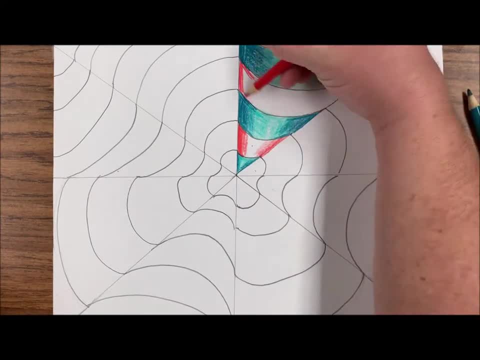 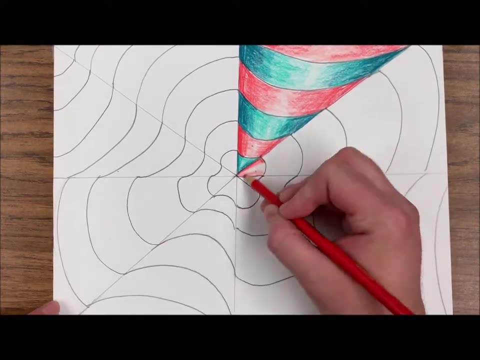 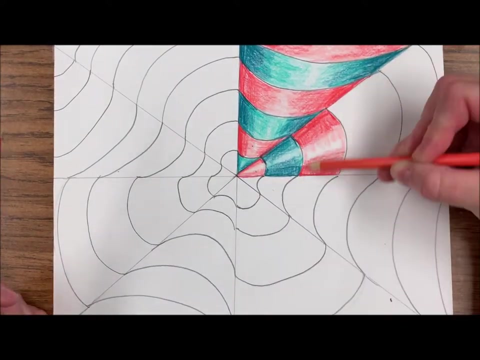 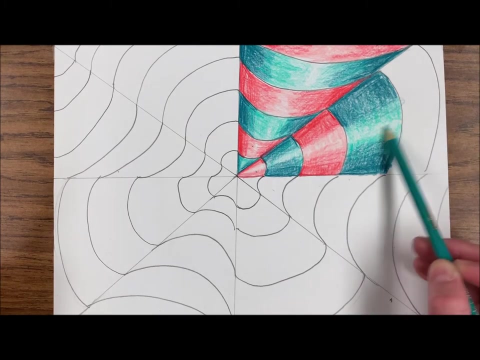 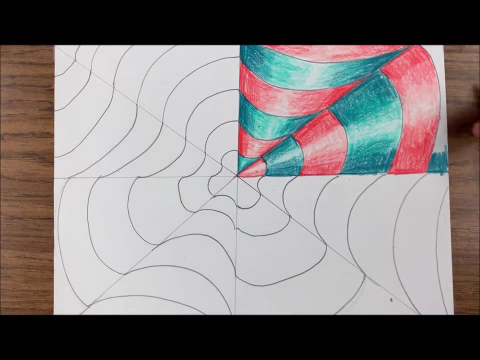 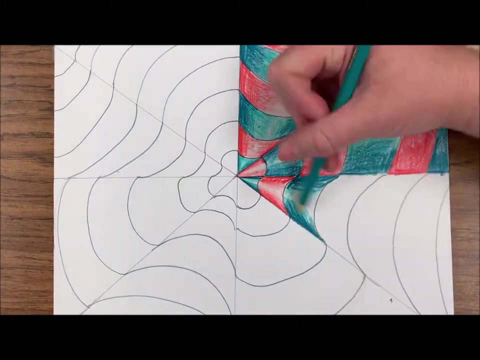 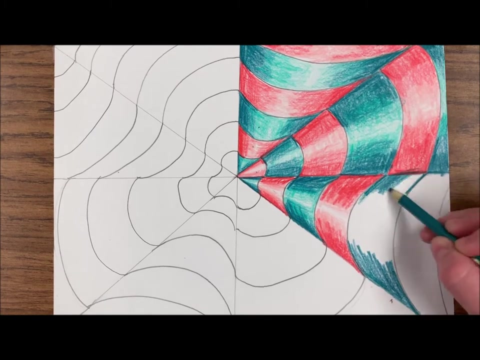 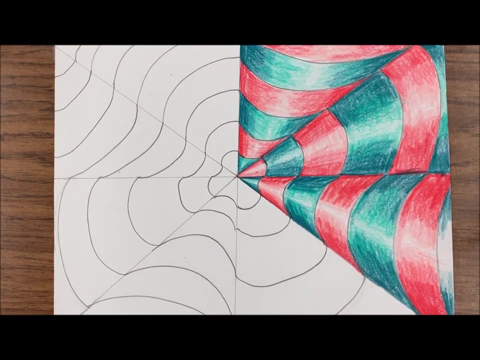 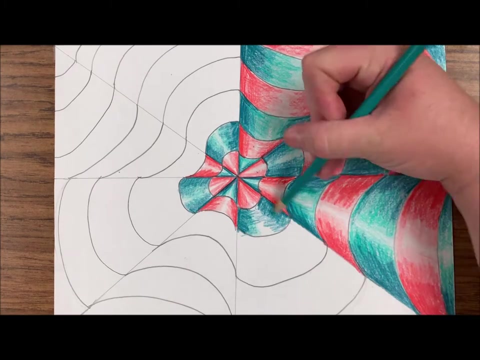 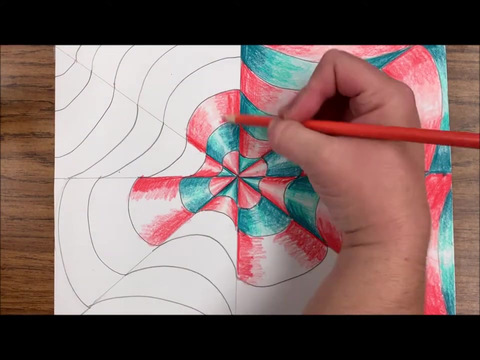 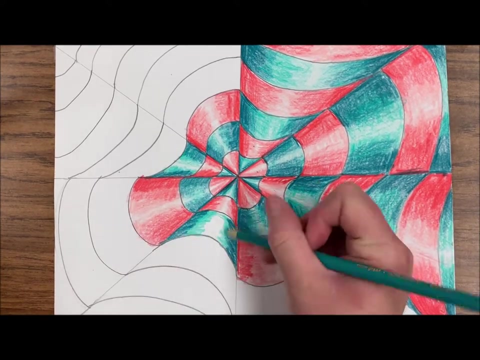 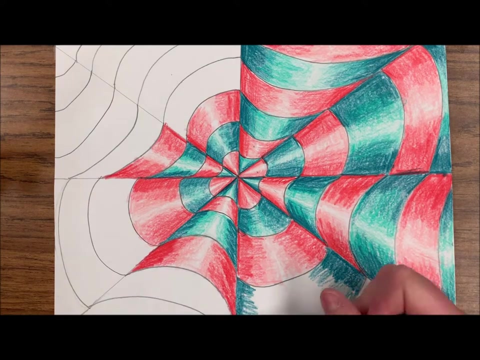 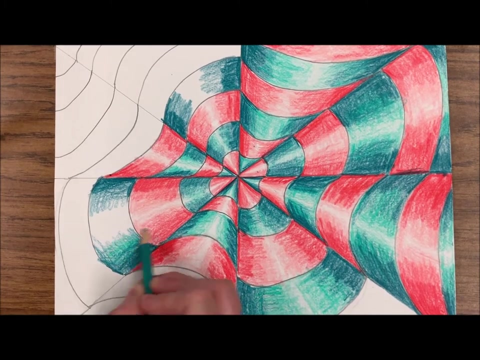 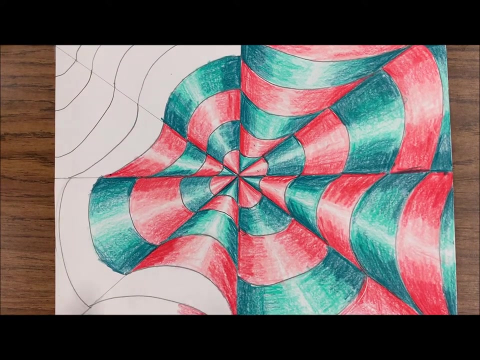 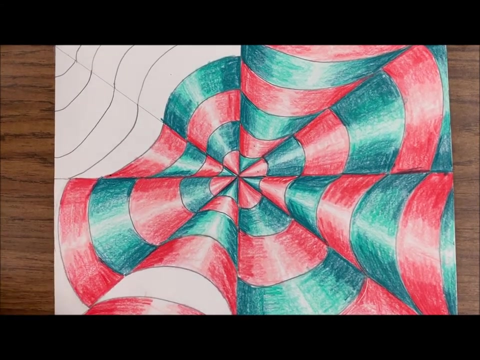 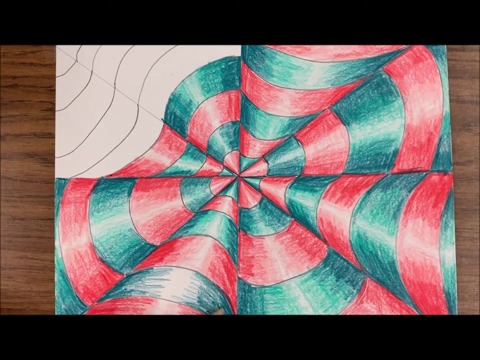 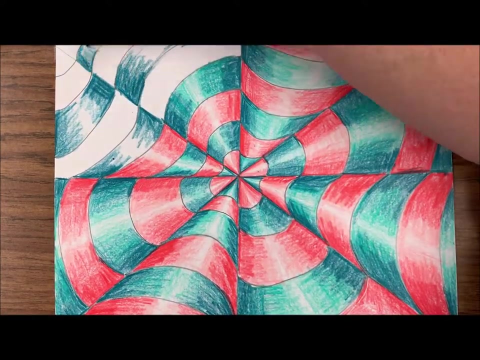 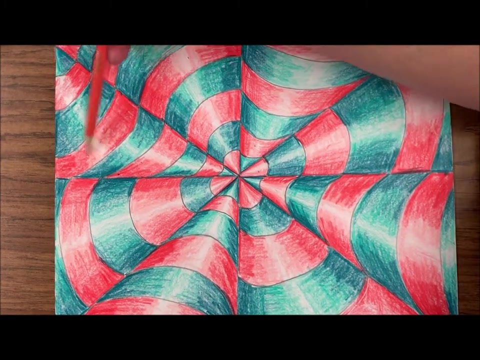 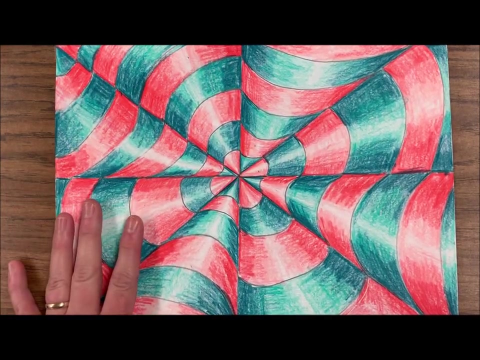 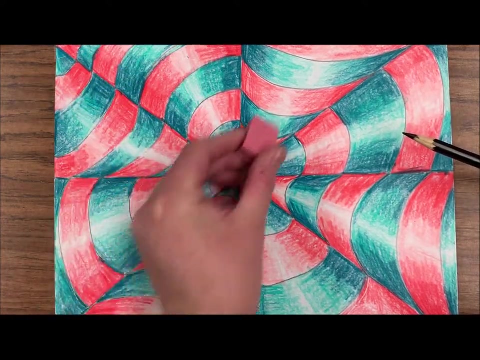 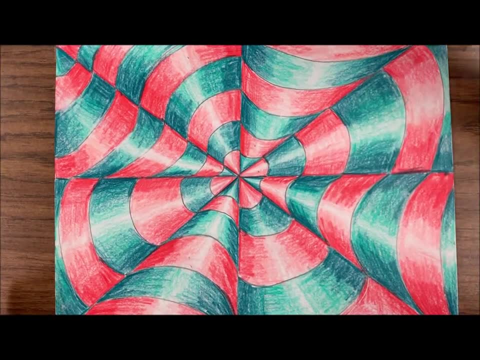 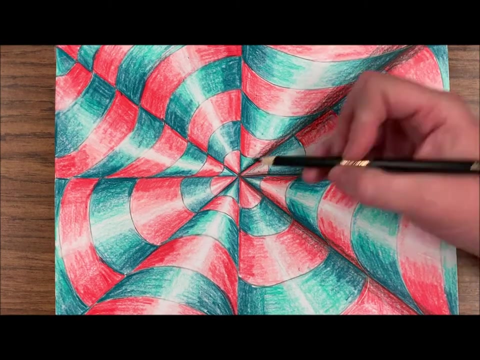 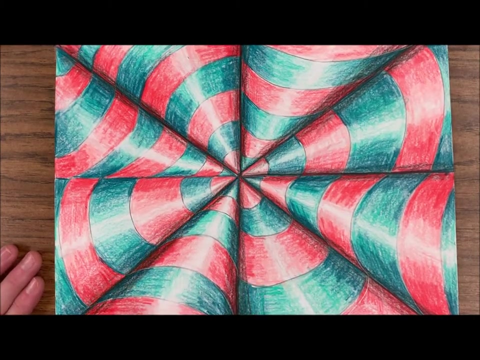 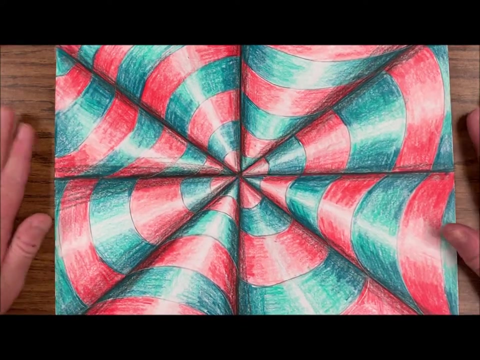 In the lines, And I'm also going to take a black colored pencil and just shade in the very edges of each cone in the crease, to really make them darken and pop. So this is my 3D optical Illusion cones using warm and cool colors. 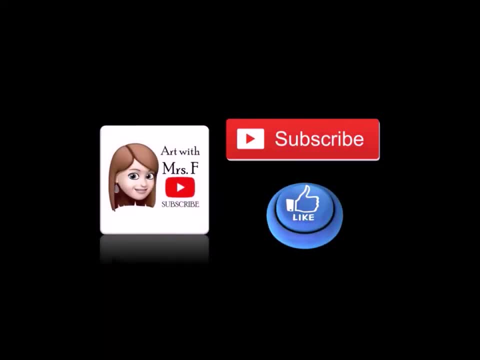 And if you like this video, don't forget to subscribe and like.